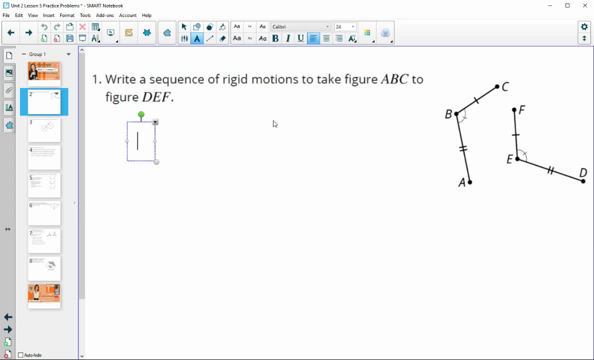 So when we're doing this, we will just want to get these touching. So we're going to want to translate figure ABC by directed line segment and whatever you want to connect. I'm going to go A to D, So by directed line segment- A, D- Then we will rotate the image of ABC. 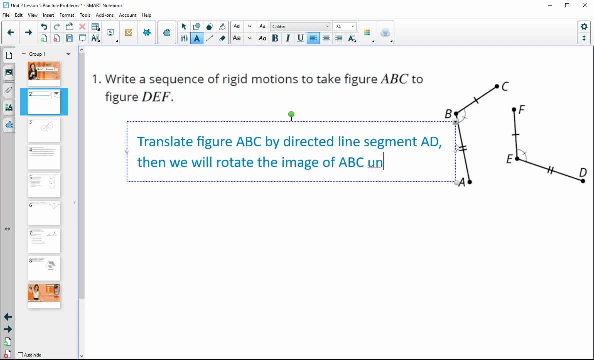 Until we will rotate the image of ABC until the image of B coincides with E. So we're going to take this, We're going to move it over here. So let A lands on D, Then we're going to rotate that image until the image of B lands on E, And then everything lines up. 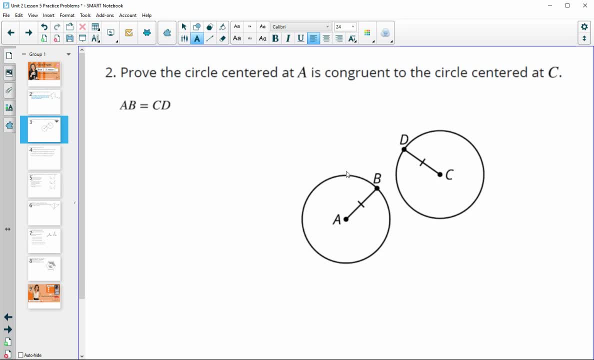 Number two: prove that these two circles are congruent. So prove that circle A and circle C are congruent. And they tell us here that the length of AB equals the length of CB. So we know that segments AB and CB have the same length. So that means they are congruent. 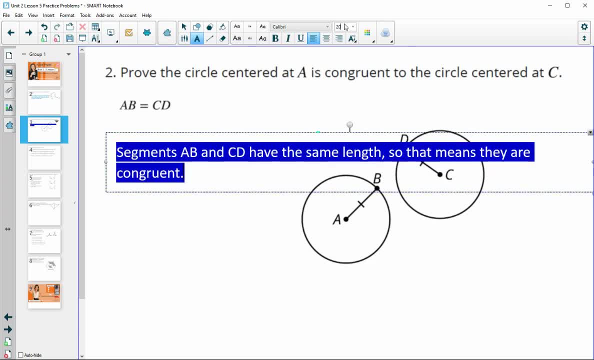 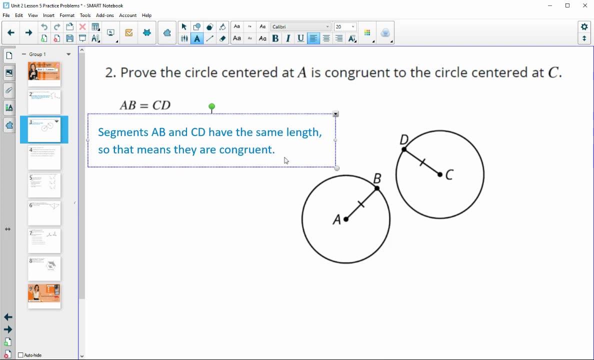 to one another. I'm going to make this a little bit smaller here- And the reason it's important that we know that they are congruent to each other is then we know that we'll take one to the next. So if these are congruent, therefore, there is a rigid motion that 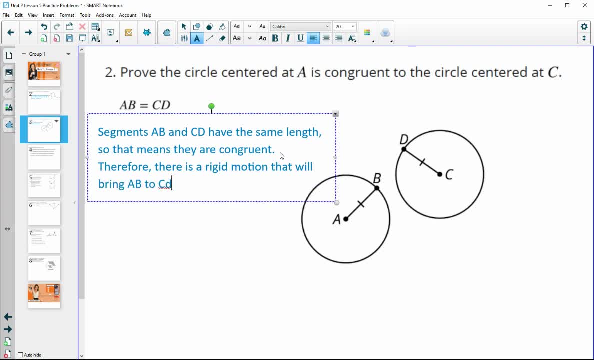 will bring AB to CB, So we will apply that rigid motion. So now we've gotten segment AB on to CB. Then we know the definition of a circle And then we know that snail size versus the length of AB equals the length of B. 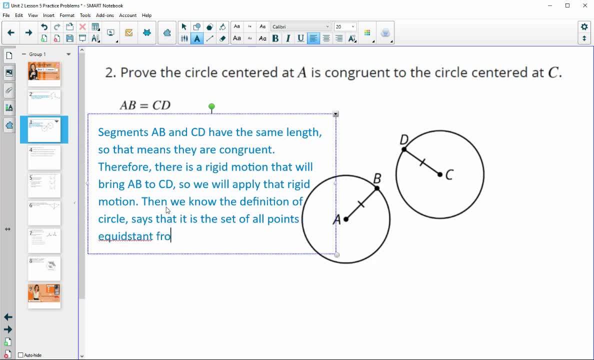 This is the set of all points, And this says that it is the set of all points equidistant from a given center. So that means that one, two, three, four, five, six, seven, eight, nine, 10, and 20 are equal to the length of AB. then that means that if we think about, the length of AB equals the length of B. we know that it's the set of all points, that is the set of all points, And so that's the set of all points. 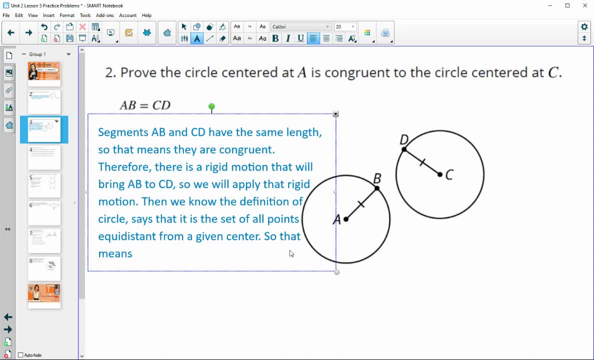 so that means that one circles center and radius. so now, if we know that it's this, the circle is the set of all points equidistant from the center, and we know that these two radii are the same. so that means that one circles Center and. 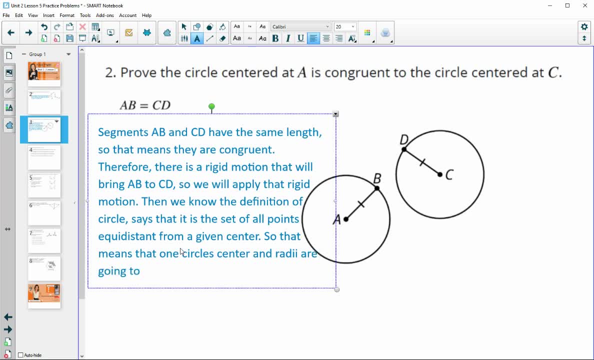 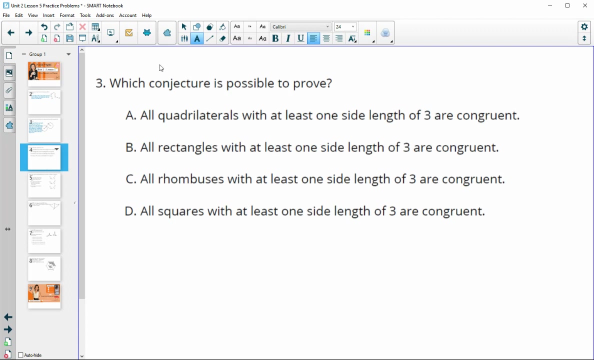 radii are going to coincide with the other circles- Center and radii- then therefore we get all of the points will land on the other one and meaning that they're congruent. number three: which conjecture is possible to prove? and so to prove that it's true. 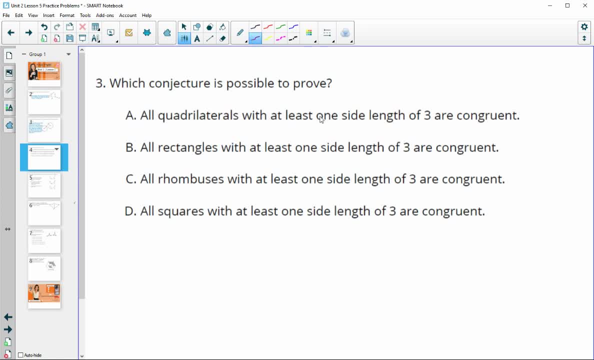 so a says all quadrilaterals with at least one side length of three are congruent. so every quadrilateral that has a side length of three are congruent is what this is saying, and that's false because this could be three, and then these could be all sorts of other things and we could have something like this: 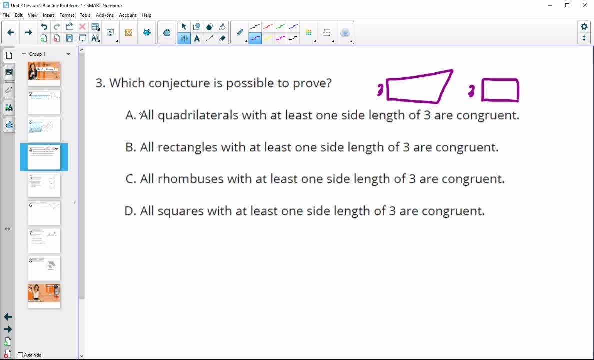 with this one being three, and this and those are clearly not congruent. so that's called a counterexample to show that that's not true. all rectangles with at least one side length of three are congruent, and so we could have something like this where this side is three, so we would. 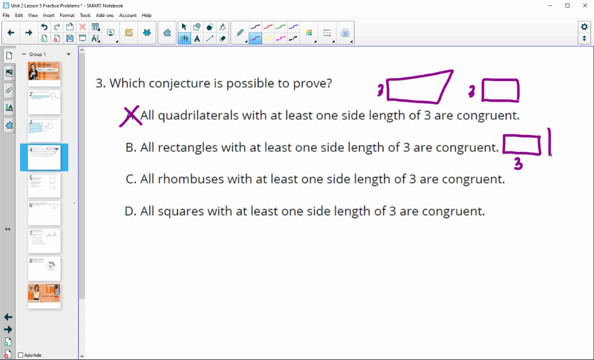 know this one is, but that doesn't mean that it's gonna be equal to the others, because we could have this with three here. so these two would be three, but these could be four and these could be one. so that's false. all rhombuses with 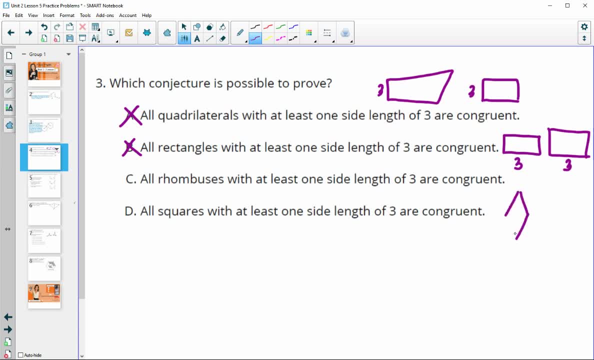 at least one side length of three are congruent. so now we know all of the sides are gonna be three, so every single side here is three. but rhombuses don't have set angles, so it could let me try and make one that looks fairly different than that, so like this could be a much skinnier angle at. 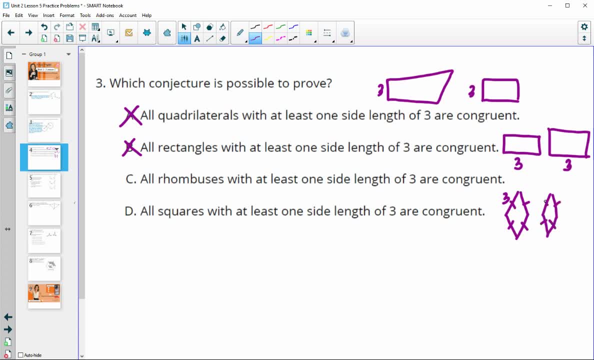 the top and all still have three side lengths, but definitely not congruent rhombuses. so this one must be true: all squares with at least one side length of three are congruent, and this is true, and we would know that because this is a square has set angles, so all of the angles in the square are 90 and then all. 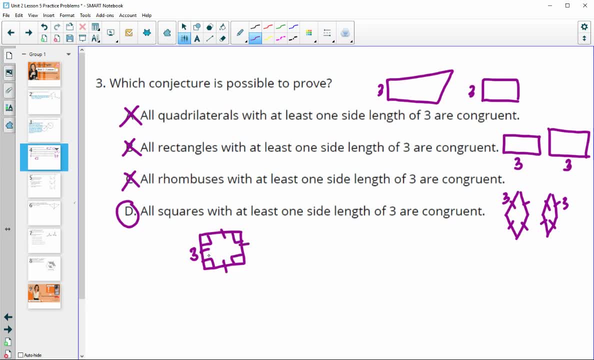 of the sides are the same, so all of these are three and all the angles are the same, and so if you draw another square, it's gonna have to have 90 degree angles, and if one of the sides has to be a three, then all of the sides have to be. 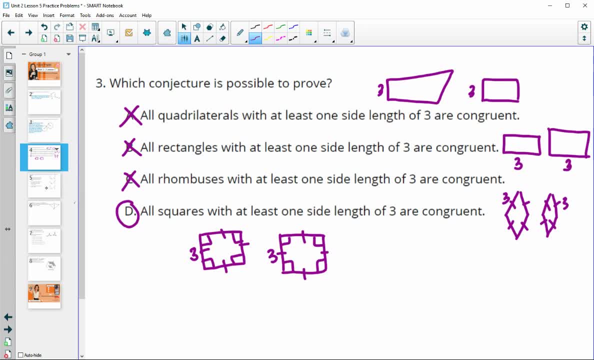 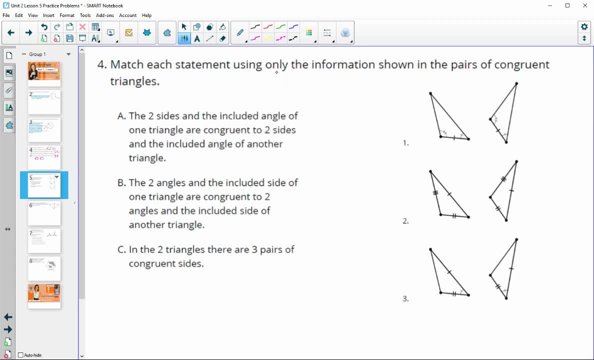 a three, since it's a square, so D would be true. we would be able to prove that one number four match each statement with using only the information shown in the pair of congruent triangles. so which pair of triangles- one, two or three- shows two sides and the included angle of one triangle is congruent to two sides. and 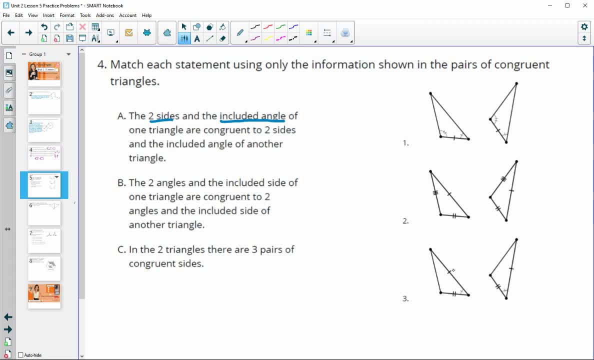 the included angle of another triangle. so we want to see two sides marked and so we see that down here. number three: two sides included angle. two sides included angle. so this one is number three. B says two angles and the included side. so we're looking for two angles and the 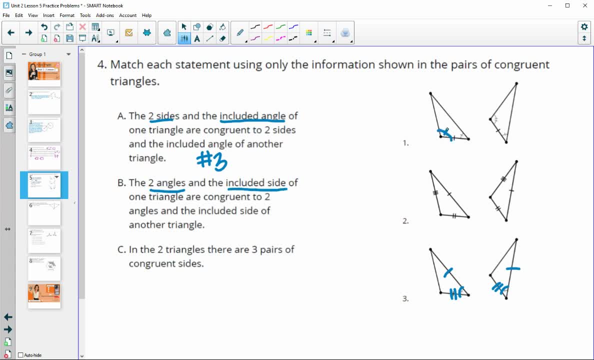 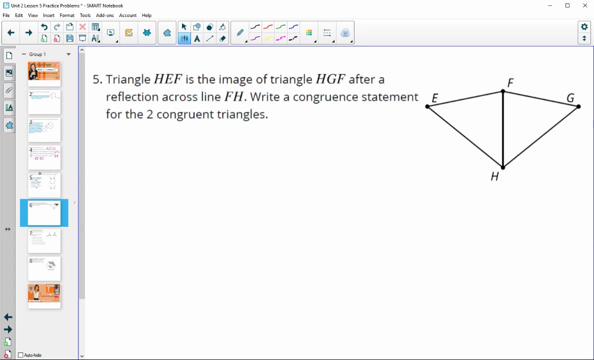 included side in one triangle, so two angles and the included side in one triangle congruent to two angles and the included side in another. that's represented in diagram number one. and then C has two triangles where there are three pairs of congruent sides and we see that in number two, number five, two. 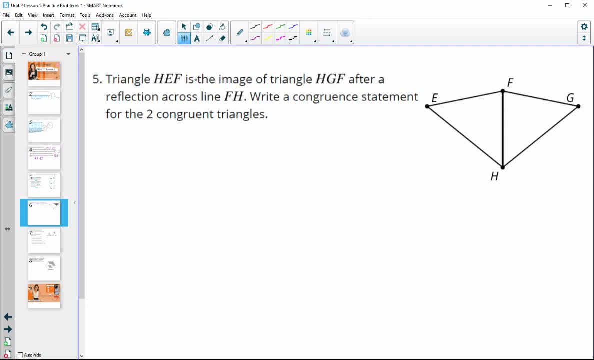 three aviators are one, a one, two and three. so those are the two triangles that we need to be congruent to now. next we're going to look at triangle H E- F is the image of triangle H- G- F after a reflection across the line F- H. so we've 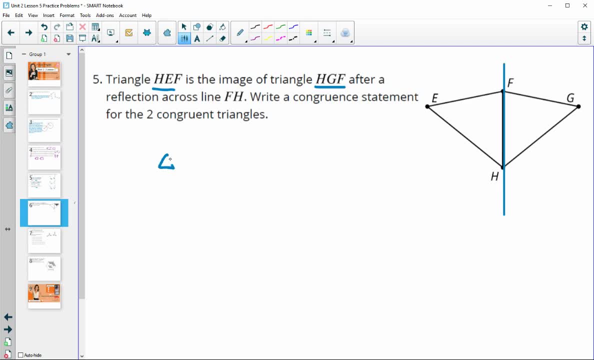 got a reflection here and it just says: write a congruent statement for the two triangles. so since they're saying these are images of each other, they must be congruent. so you could just kind of steal that and just put triangle H, E, F is congruent to triangle. 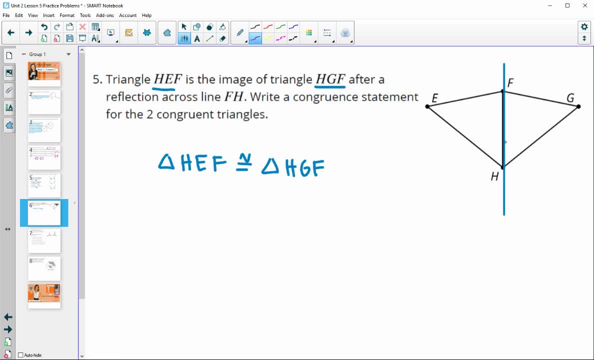 go to the picture and do it in a different order if you wanted. So, if you wanted to go H- sorry, F H E- you could do that. So F H E is congruent to, and then just follow the same. 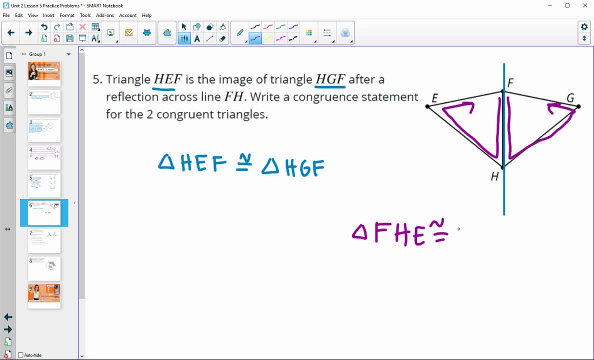 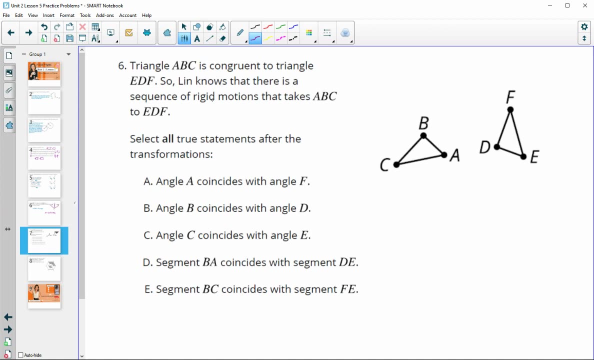 order on the other side. So F, H, G or there's some other options too for you, but there's two. Number six, triangle ABC is congruent to triangle EDF. So Lynn knows there's a sequence of rigid motions that takes ABC to EDF. Select all true statements after the transformation: 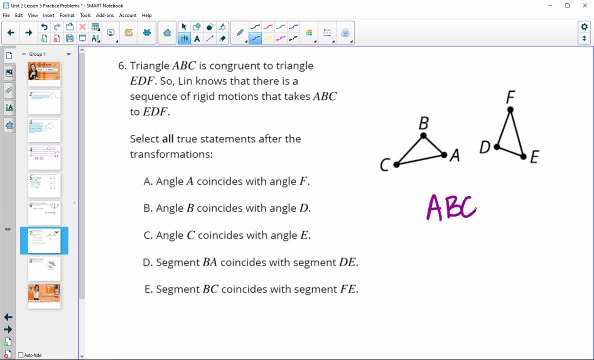 So I'm just going to write these two congruent triangles out a little bigger. So we've got ABC and then we've got EDF And I'm just going to line them up with each other so we can kind of see the course pattern. So I'm just going to write these two congruent triangles out a little bigger. 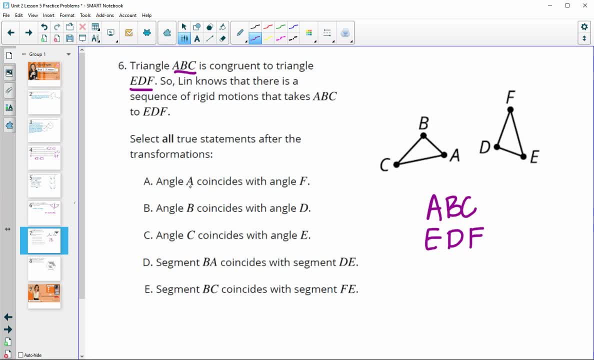 So A says that A is going to coincide with F, and that's false, because A is going to coincide with E. B is going to coincide with D. that's true. C is going to coincide with E. that's false, And I like to do it this way because these triangles look pretty similar. They'd be easy. 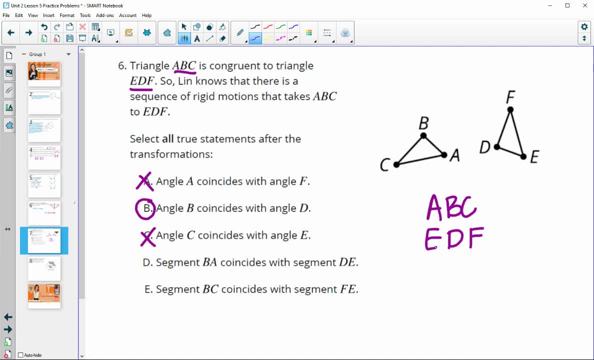 to kind of screw up if you're going by looks. So when they tell us which two triangles are congruent, it's nice to look at the order of those letters. Segment BA- so these first two letters- is congruent to segment FE, which is the first and the last. So that's going to be false. 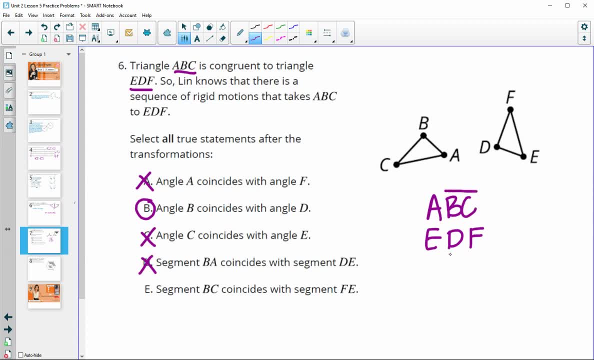 And then segment BC. so the last two letters is going to coincide with FE. Oh, whoops, I read that one wrong on the last one, So I read this one instead of this. Okay, so let's look at D again. So BA with DE. Okay, 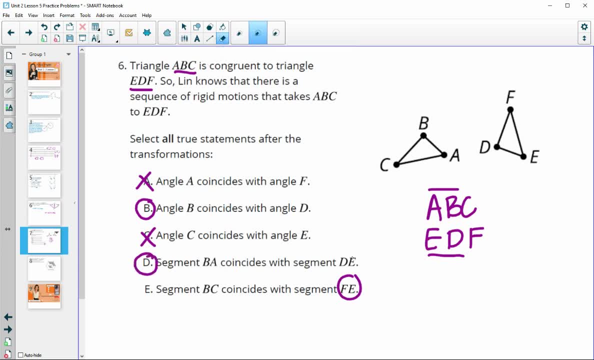 first two and first two. So this one is actually true, And then this one. BC coincides with FE. So BC is these last two and then FE is the first and last. So that one's going to be false. Sorry about that. 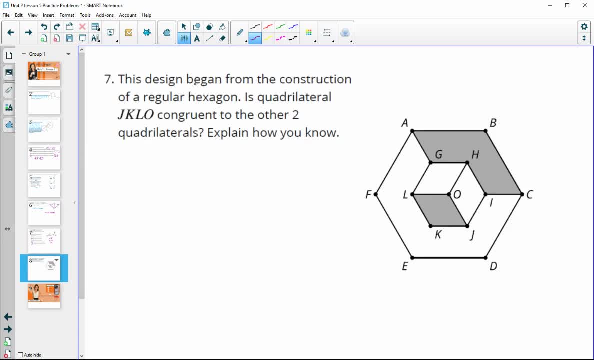 And then number seven. this design began from the construction of a regular hexagon. So we know all the sides and angles are the same. Is quadrilateral JKLO. so this shaded quadrilateral here. is this congruent to the other two quadrilaterals? So is it congruent to this one?